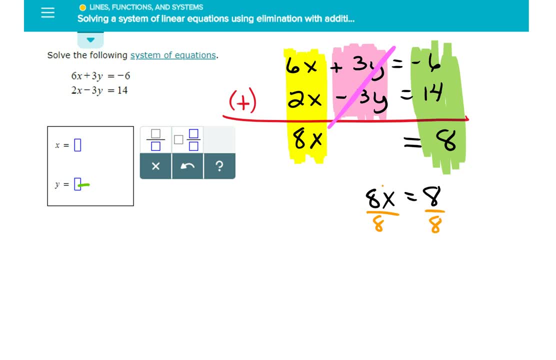 And then I'm going to divide both sides by 8 to figure out what x is. Of course, 8 divided by 8 is 1x, And 1x is 1 times x, which is just x Equals. 8 divided by 8 is 1.. 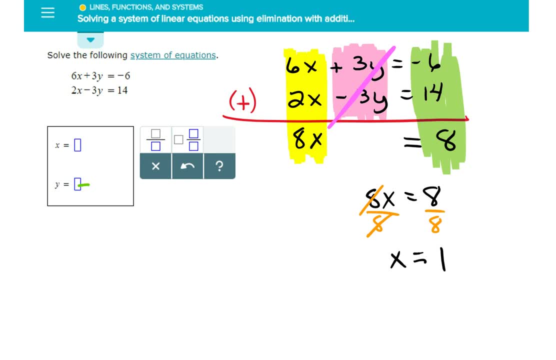 I don't know if you noticed this, but when I went to add them together, everything has to be lined up. The x's are lined up, The y's are lined up, The equal signs are lined up And the constants, the numbers that have no variables, they're called constants. those are lined up. 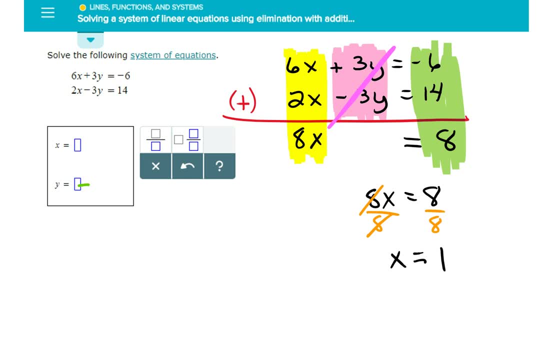 So everything is lined up with its like term. Now, once you get, x is equal to 1, they're not going to make you go back and do elimination again. You are simply going to take this answer for x And you're going to take it back to either the top equation, where x is, or the bottom equation, where x is. 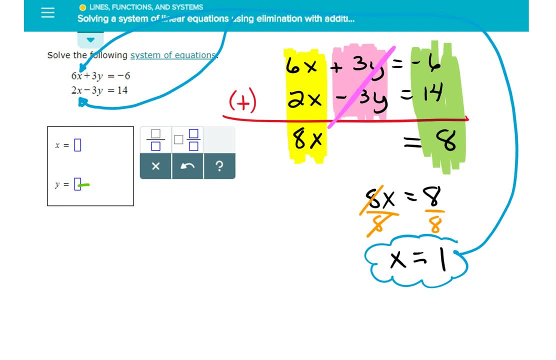 It really doesn't matter. You are solving a system of linear equations. That means if I graphed these, they would be straight lines and they would cross each other at the point with coordinates. of x is equal to whatever I just got, which was 1.. 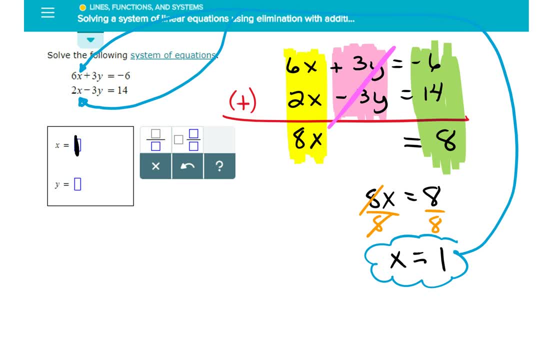 Right, x was 1,. there's my first answer, And then I'm going to plug and chug the 1 into the equation to get the y coordinate. And it doesn't matter, You can use the top one, You can use the bottom one. 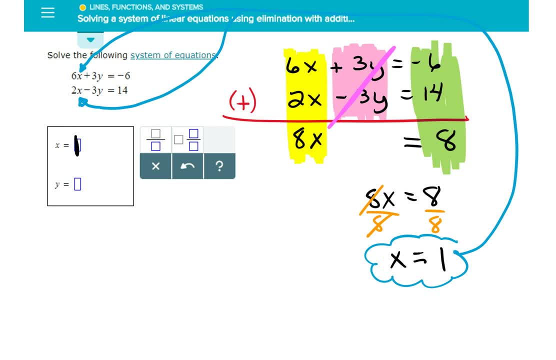 They're both going to work. For the top one it would be: 6 times x is 1 plus 3y equals negative 6.. 6 times 1, I'd start here- That's 6.. And then I'll start solving. 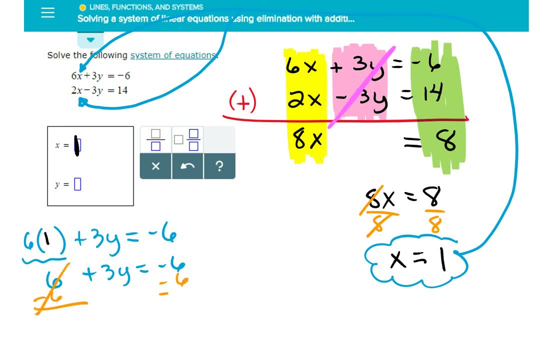 I'm going to subtract 6 to cancel that out, But I've got to subtract 6 from the other side. What you do to one side of an equation, you have to do the same thing to the other. You've got to keep that equality. 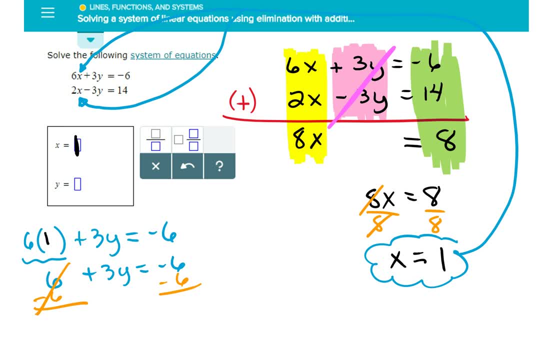 It's just like a scale: If you take 6 pounds off one side, you've got to take 6 pounds off the other to keep it in balance. So I'm left with: 3y is equal to negative 6.. Take away another 6 is negative 12..